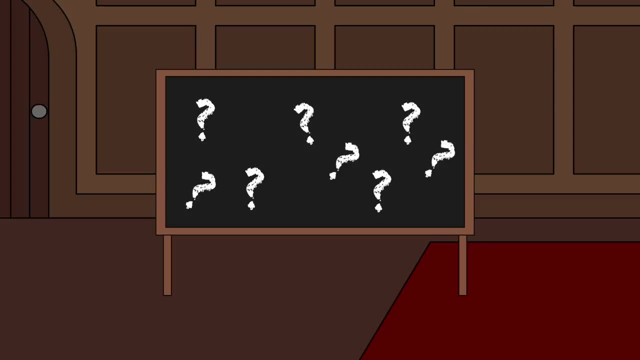 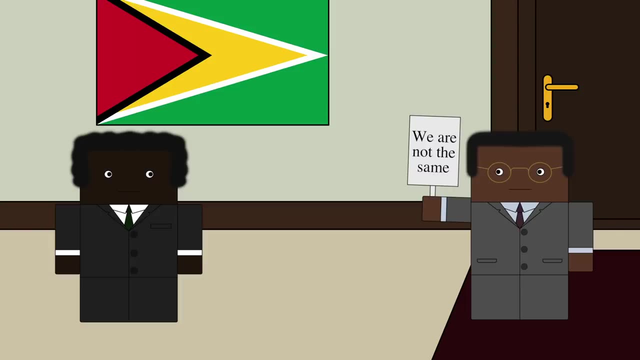 But why is this the case? Why are there so many countries with Guinea in their name? So, before we answer that, there's something that needs to be cleared up: The Guineas and the Guianas are not related: Two different words with two different histories. 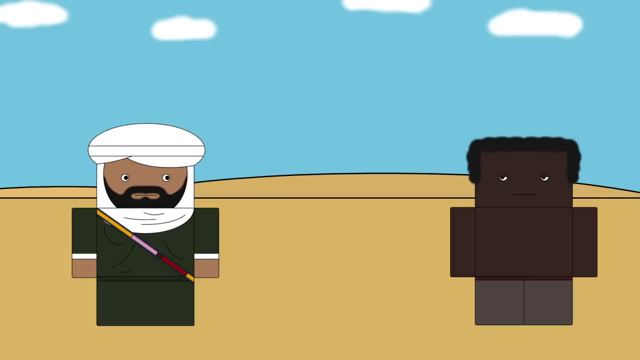 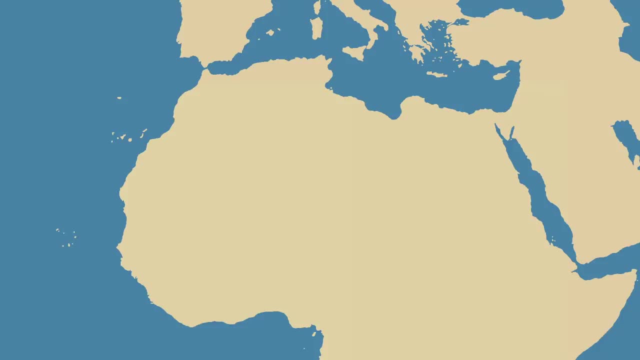 The one we're focusing on most likely comes from an old Berber word which means dark skin, And it was used to describe the collective lands along the coast to their south and the people who lived there. Europeans only had a few names for parts of Africa. 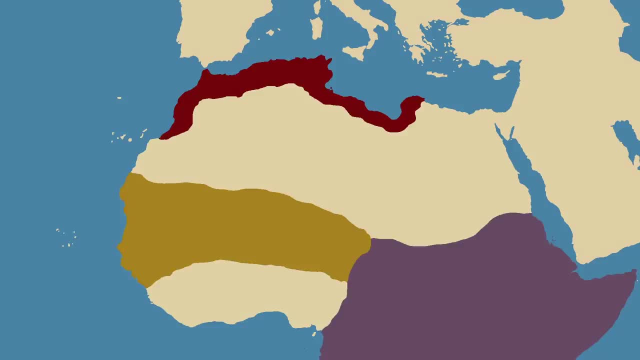 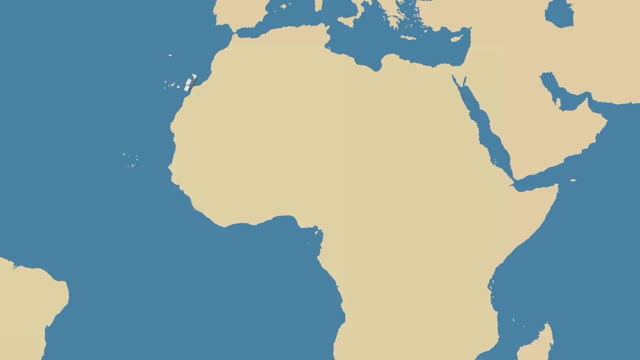 like Barbary for the north, Ethiopia for most of the continent- another term for this area- and Guinea was adopted for these lands. You see, Europeans made use of North African navigators to help them sail down the coast of Africa, and so it wasn't long until the 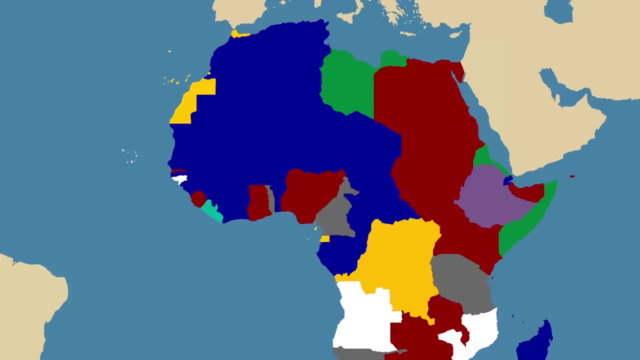 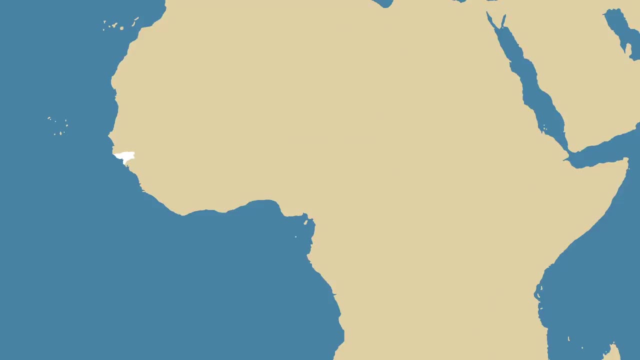 name for the region stuck with all of them, And when Europeans later colonised the area, the different European powers used Guinea to refer to their separate parts of it. The first was Portugal, who claimed this area, calling it Portuguese Guinea. There was also Swedish Guinea, which would later become Danish. 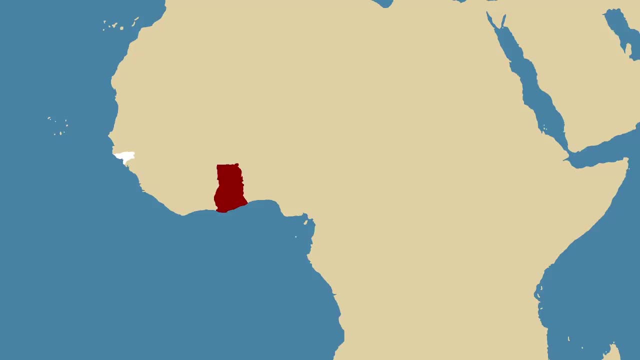 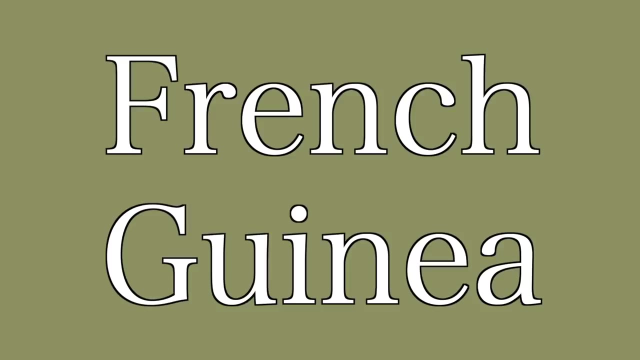 Guinea and, soon after that, Dutch Guinea, before the British took it for themselves and called it the Gold Coast. In the late 19th century, France had its turn to colonise parts of the area and, in a shocking display of originality, called it French Guinea. Later, when decolonisation, 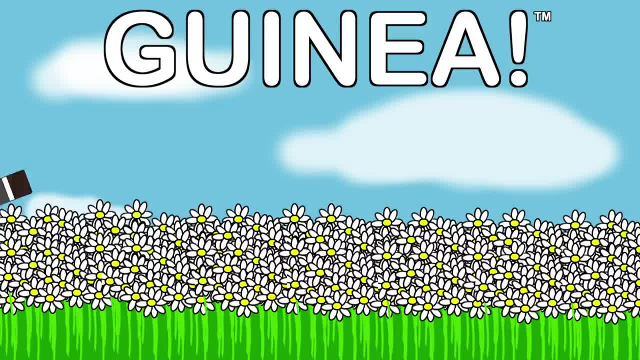 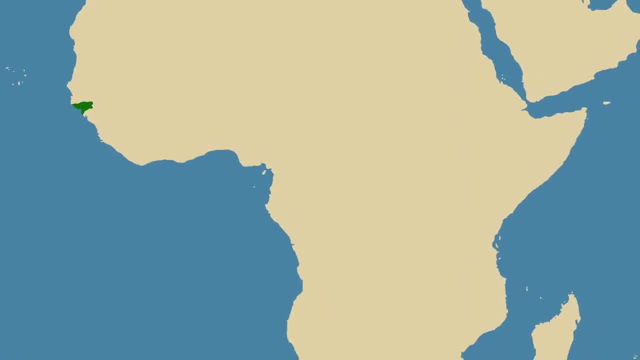 saw Africa freed. French Guinea was the first to win its independence, and so it got dibs on plain old Guinea. About 20 years later, Portuguese Guinea followed, and it soon took the name Guinea Baisal. To the south, mostly outside of the region, is Equatorial Guinea. This was first. 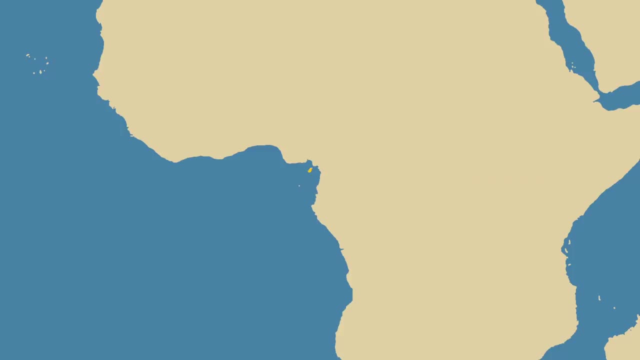 colonised by Portugal, who soon sold this island to the Spanish, who soon took control of this region. In the late 19th century, the French muscled in on this region and they signed a deal with the Spanish which settled on these borders, with Spain gaining the small colony of Riomuni, which 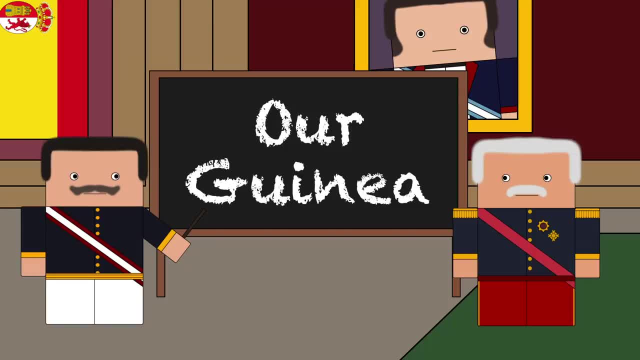 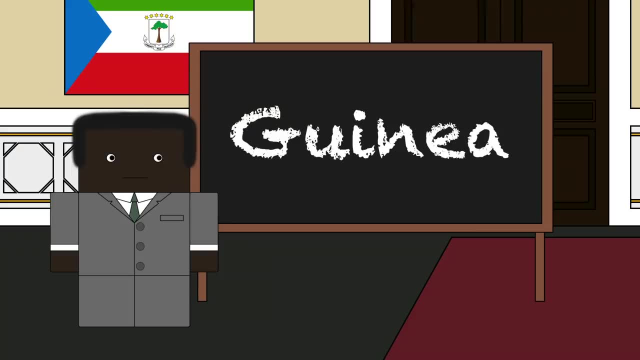 combined with the island of Bioco in 1929. And it called this combination Spanish Guinea, because the island of Bioco was a part of the region, despite the rest not being so, And when the nation gained its independence, it kept the name Guinea, but given that Guinea was already taken, 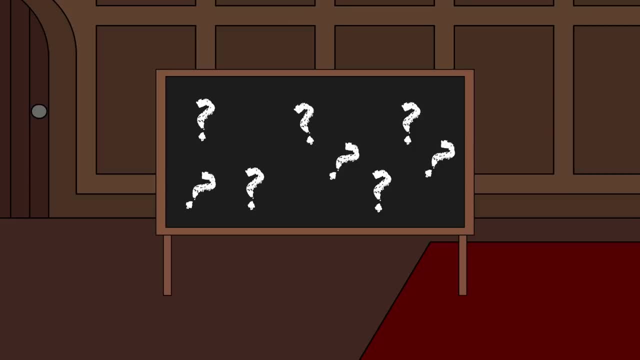 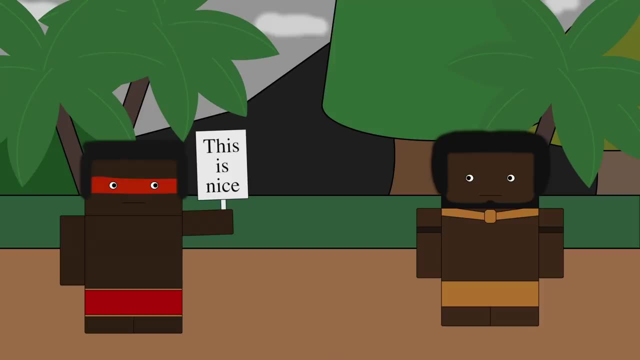 it adopted the name Equatorial Guinea because of its location. So what about Papua New Guinea, On the other side of the world, which is firmly and entirely not within the region of Guinea? Well before Europeans arrived, the island was known as Papua, but cultural sensitivity is not. 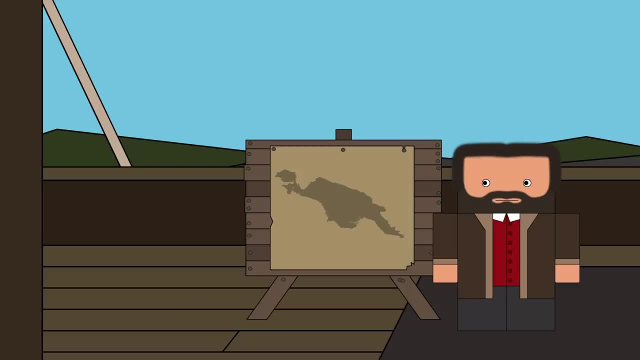 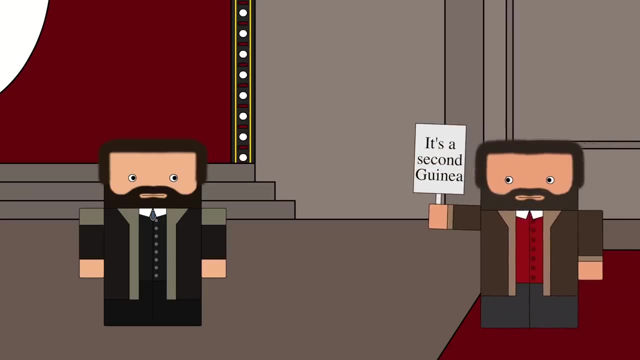 the cornerstone of imperialism, and so the Spanish explorers, who first mapped the island's coastline, picked a new name: New Guinea. So why Guinea and not something else like New Aragon? Well, they chose this name because, as far as they were concerned, the natives who lived on Papua were